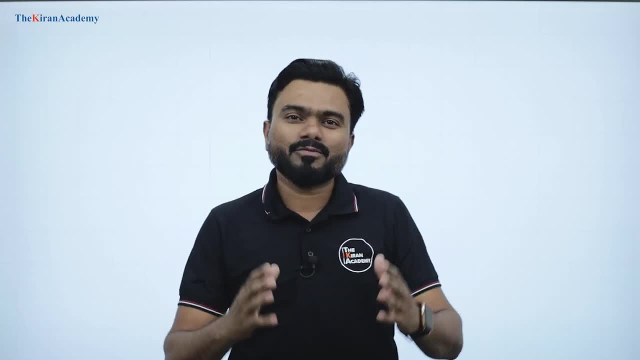 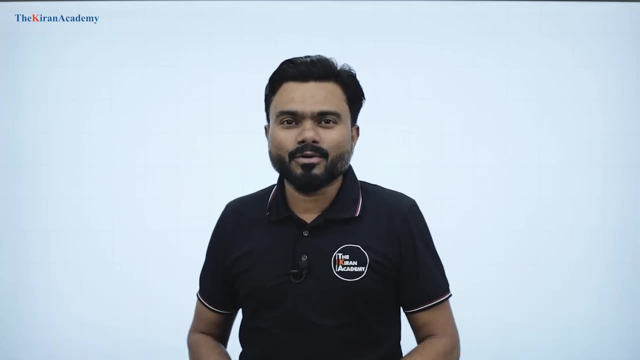 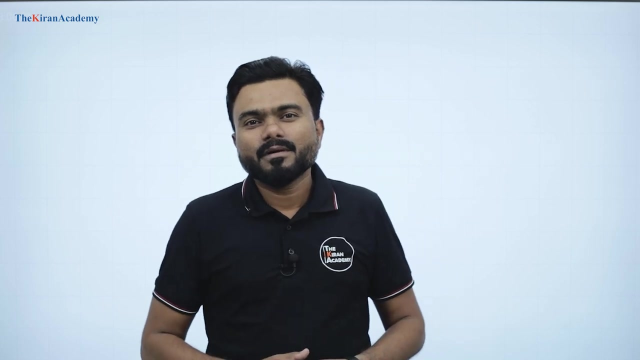 Hello guys, how are you? I hope you are doing well. and welcome to the first series of Python. So you were searching a lot, sir: which language to learn in 2024, how to kickstart my journey in Python, how to become a data scientist, how to become a machine learning engineer. So, guys, 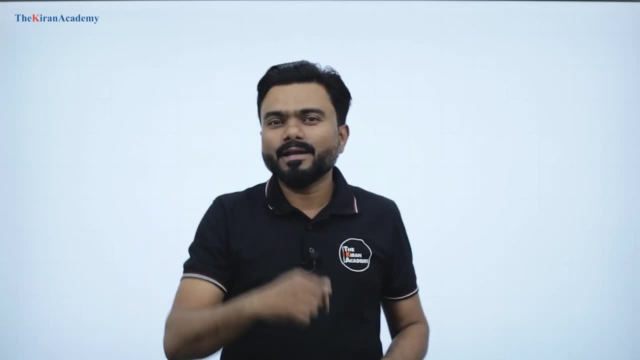 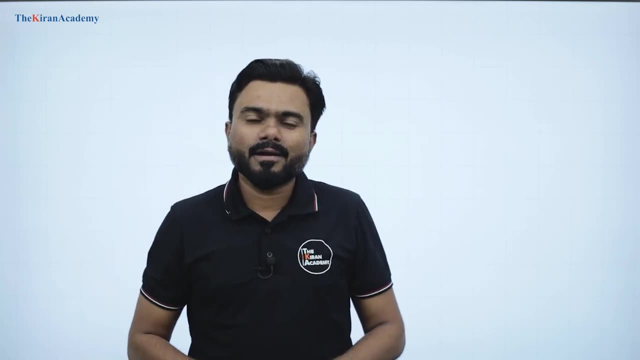 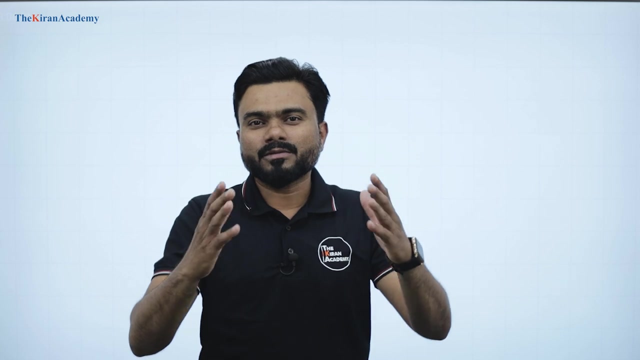 your wait is over. In this video, I'll tell you how you can use Python, what are the different applications where you can use Python and why Python is called general purpose programming language. So this is Atul, and I have 13 plus years of experience in corporate training and I have 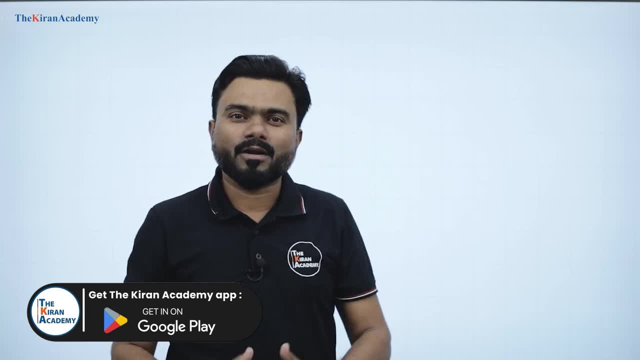 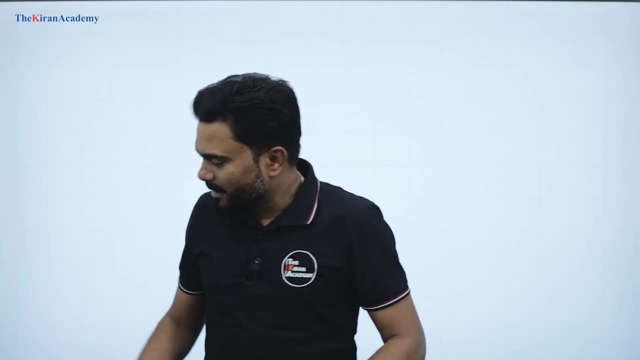 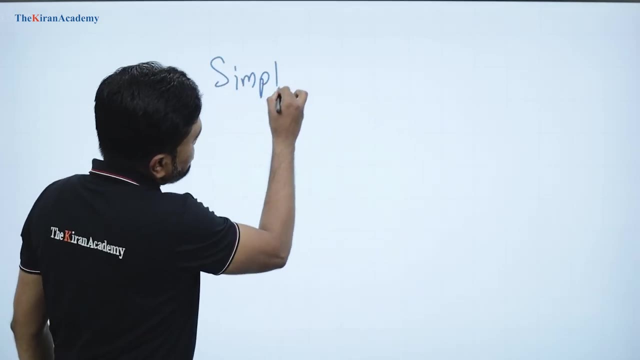 trained 10,000 plus students on Python technologies. So, guys, why to select Python in 2024?? So Python is simple programming language. So the first point is: it is simple. Why it is called simple programming language? So if you want to do the addition in Python, 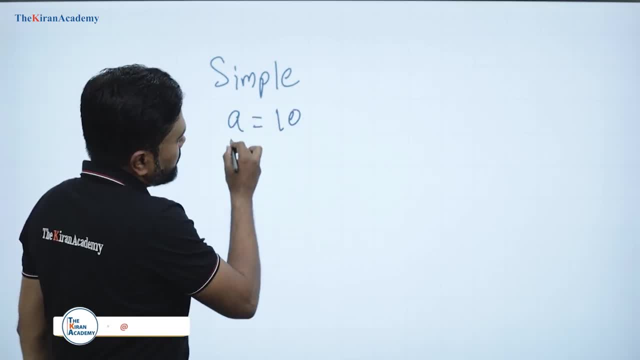 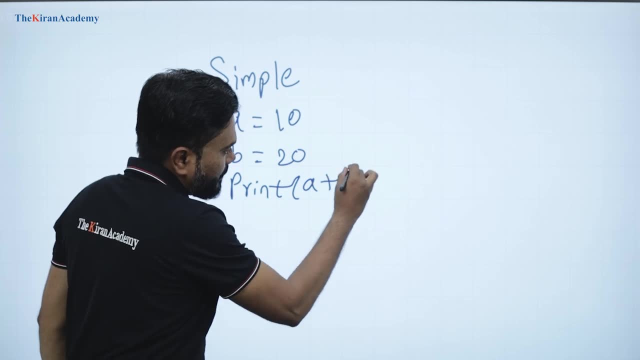 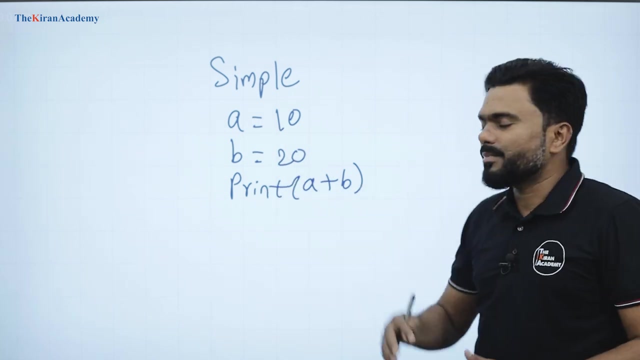 simply you define variable with some value and simply print A plus B. So for doing simple addition, you can see that just you need to declare two variables and simply print the result of the addition. So that's why, guys, Python is very simple programming language. So if you want to, 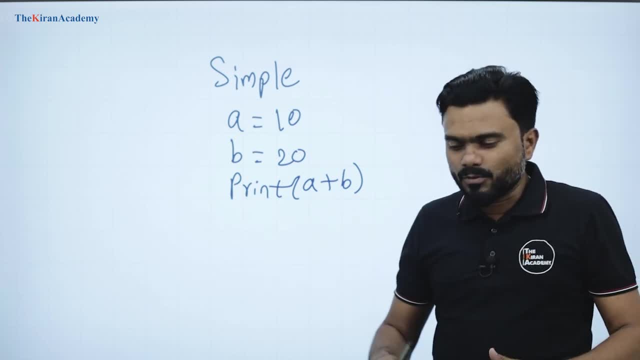 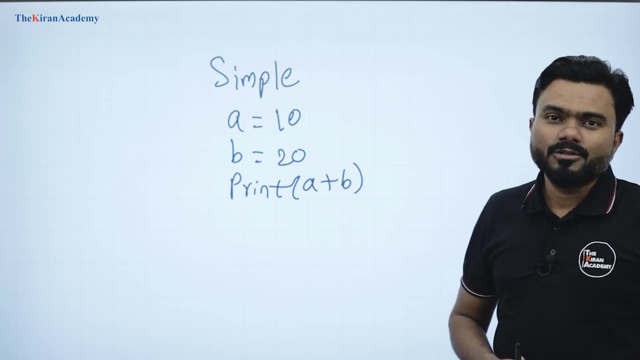 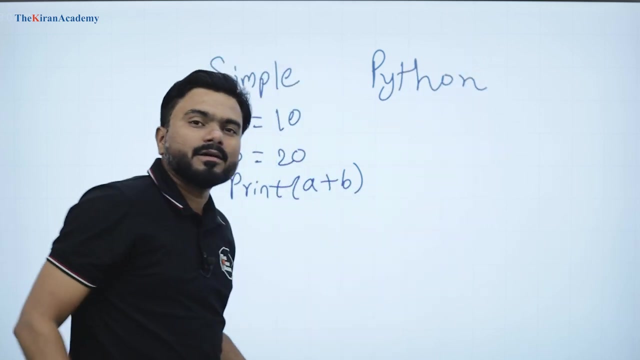 do very simple language. if you are non-IT background, if you want to migrate your career into IT and if you're stuck, how to start journey of coding? So, guys, Python is the solution. Start learning Python today itself. I'm talking about what we can do with the help of Python. 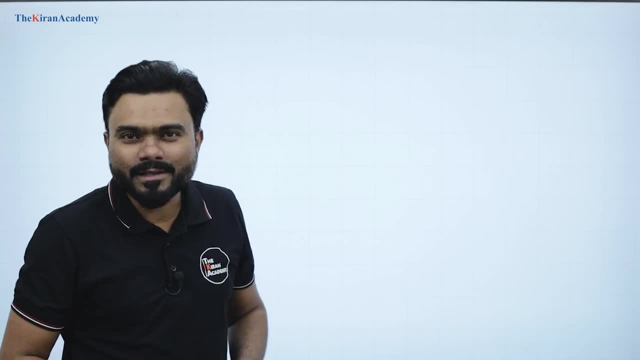 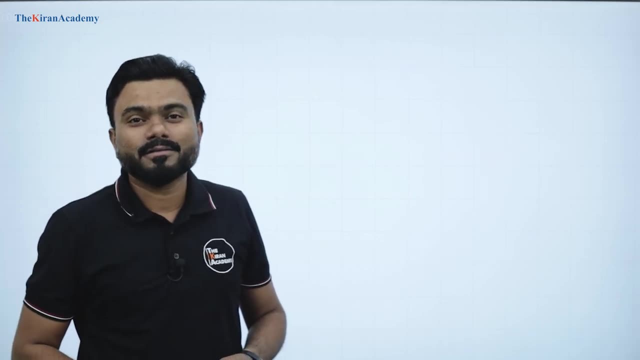 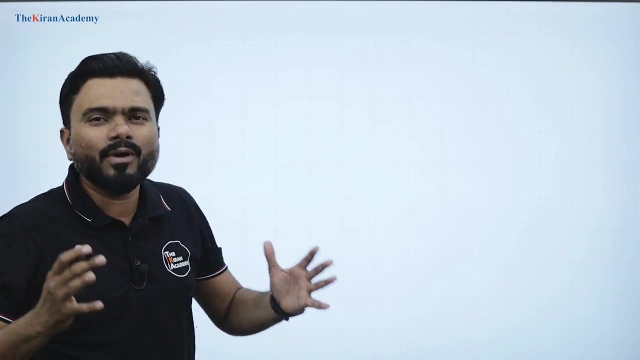 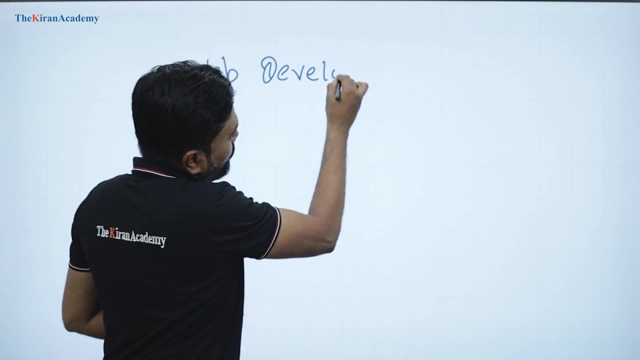 So let me tell you, guys, what you can do with the Python. Python will do the magic for you guys. How So, if you want to start a journey, you want to become a website developer? okay, So you can do web developer. you can design website using Python. There are so many frameworks, guys, available in. 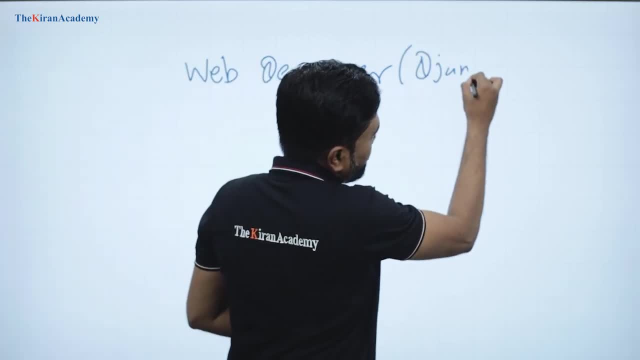 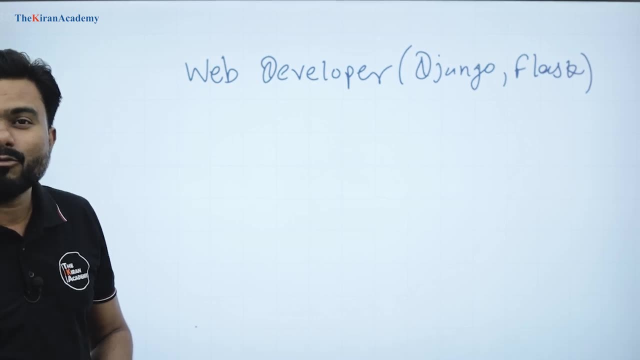 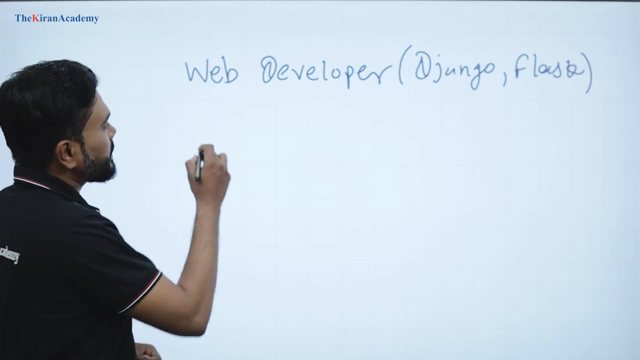 Python, like Django, Flash and many more. So learn any of the framework and you will be the Python web developer. Sir, if I don't want to become a web developer, I want to become a data scientist. You just think of the application and the solution is Python. So data. 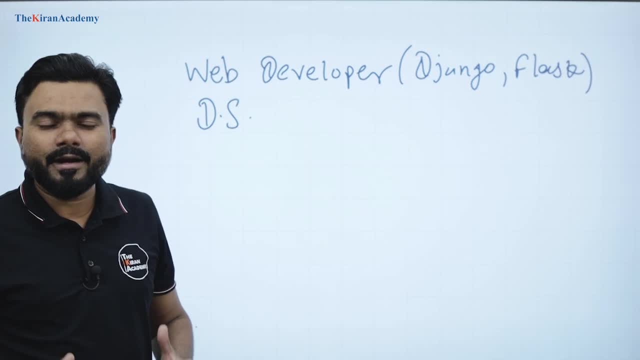 scientist, if you have to work on data, you have to process the data, guys. So industry is also telling them: choose Python wisely, Because processing of data in Python is very faster than other languages. This isn't a lie, guys, You know, just like flies or umami or……. 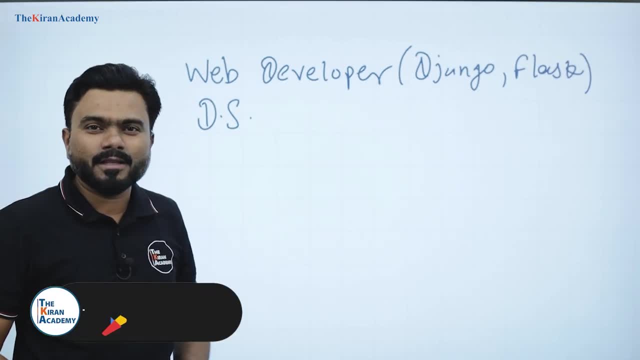 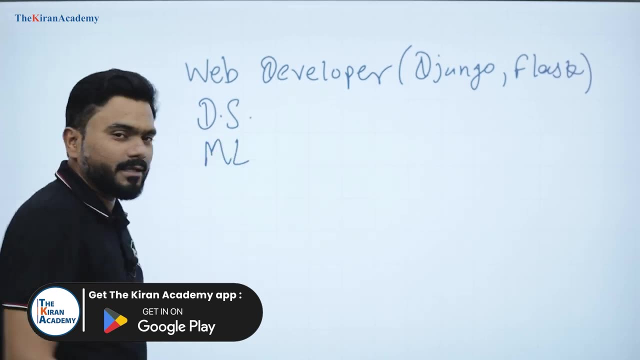 So the entire industry that wants to become a data scientist is switching to Python. Sir, I don't want to become a data scientist, I want to go into machine learning. Yes, the solution is Python, Because many people say, sir, I want to become a machine learning developer. 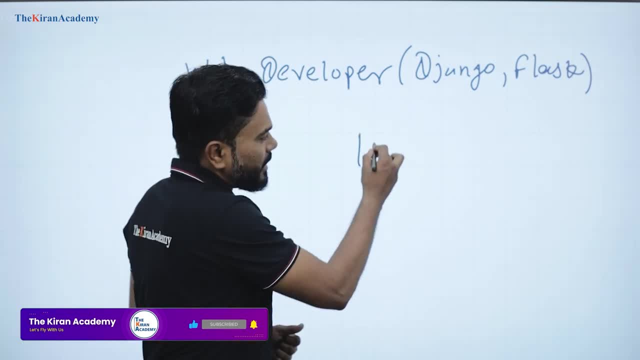 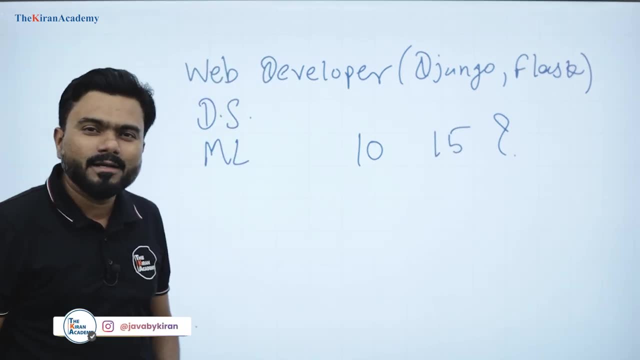 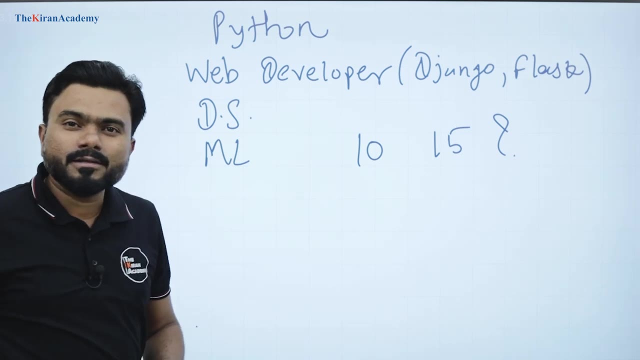 I want to go into machine learning. Packages are of 10 lakhs, 15 lakhs, But they don't know what machine learning means. So, guys, if you want to do machine learning, then please learn Python. Start learning Python syntax. 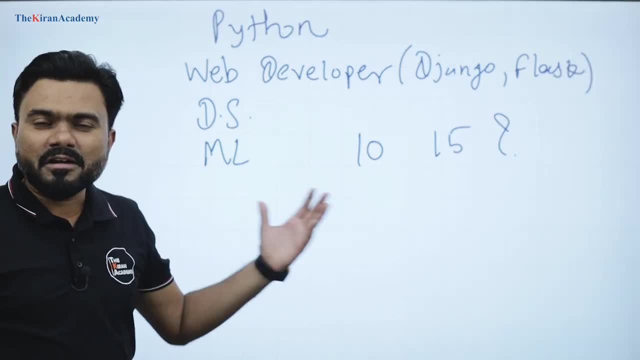 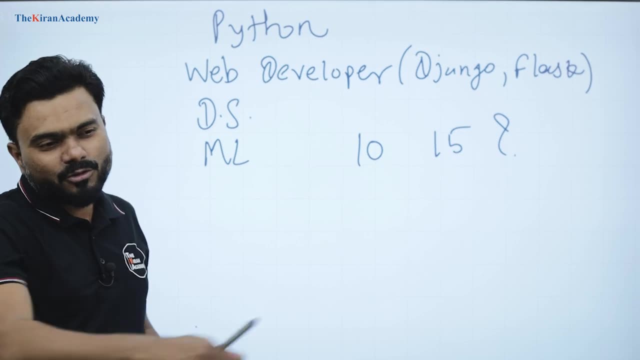 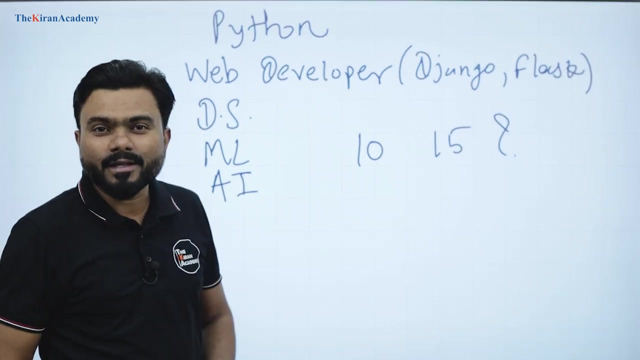 Sir, I want to go into AI, artificial intelligence. It is very trending. It is running on Google Engine AI, It is running on Gmail AI. Now it is also coming on chat GPD. So, guys, you can go into the AI also by learning Python. 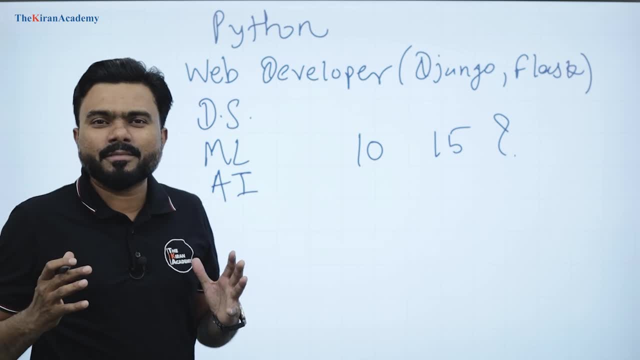 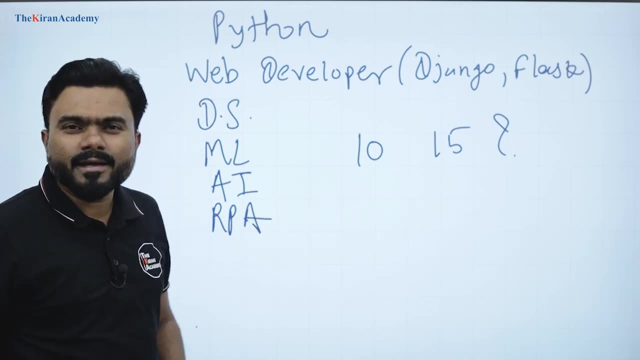 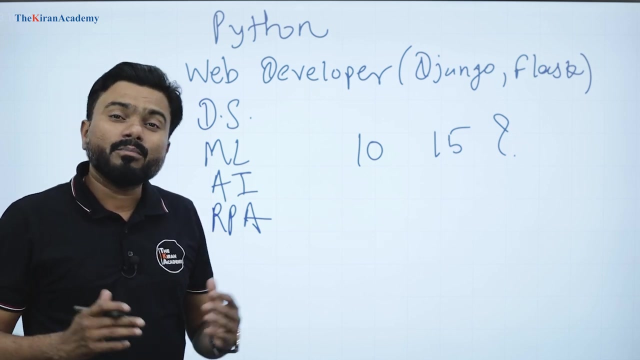 Sir, I want to go into robotics, process automation. I want to design robots. Yes, guys, RPA, robotic process automation. I have a lot of friends in the field of mechanical design And now they want to learn Python Because mechanical industry is also switching to programming. 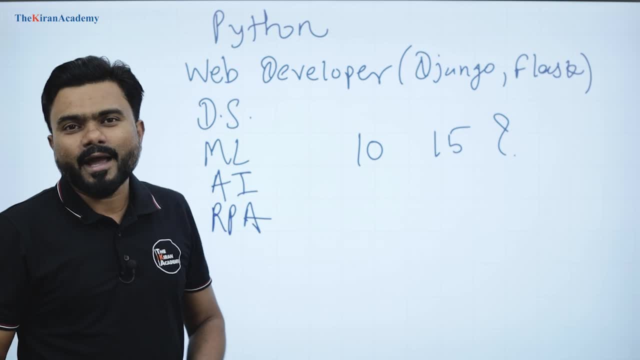 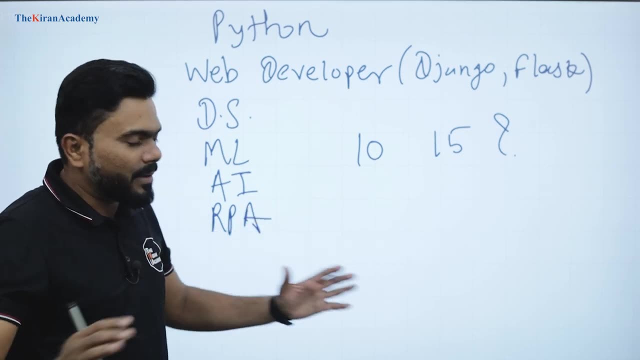 They want MATLAB, they want Python. So, guys, you can start your journey by learning Python. Sir, I want to do testing. I don't want to go into development. I don't want to go into AI, machine learning. Yes, you can do the testing.